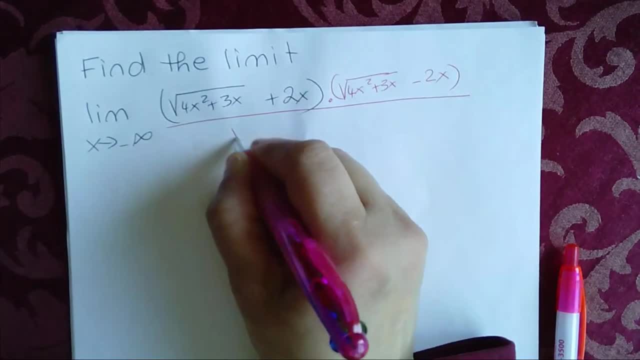 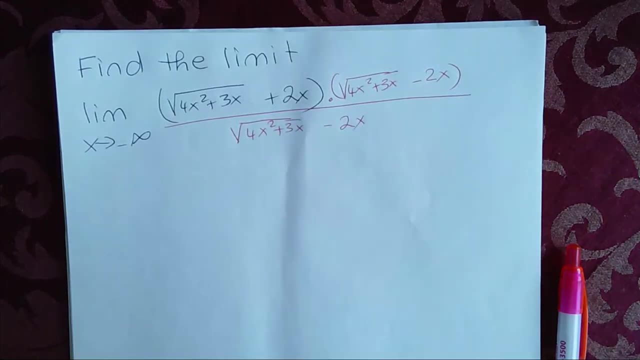 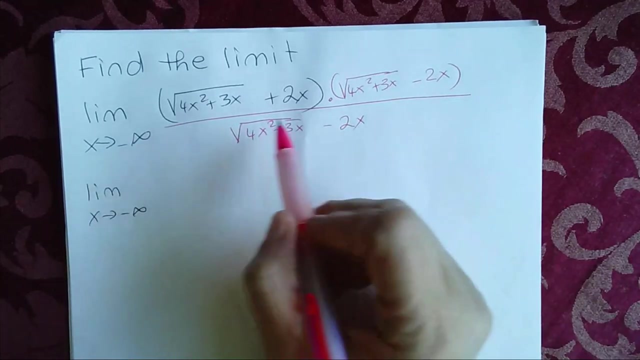 you multiply in the numerator, you have to multiply in the denominator. So square root of 4x squared plus 3x minus 2x. Now the numerator would become: this will simplify: remember: this is the product of the sum and difference of two terms. That's the same as a minus b. 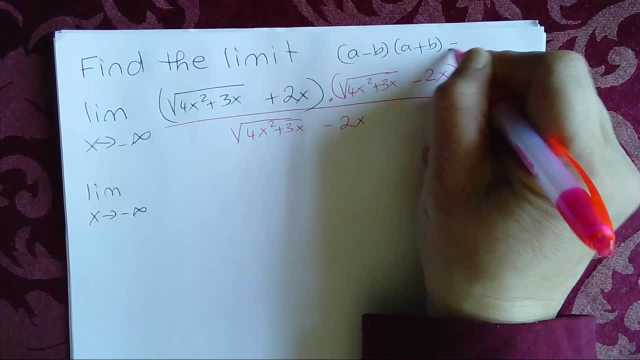 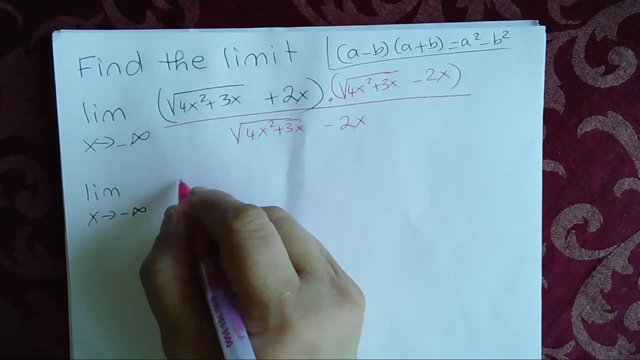 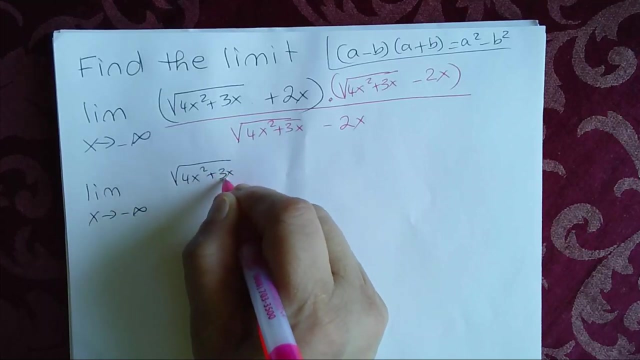 times a plus b, which is a squared minus b squared. Now, this is what we have here, And so it's the first one squared. That means that square root of 4x squared plus 3x squared minus 2x squared, divided by the denominator. 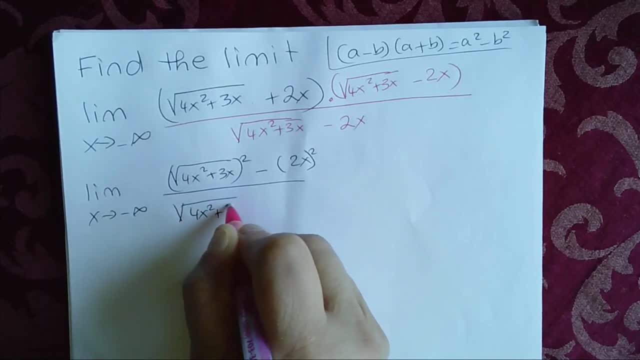 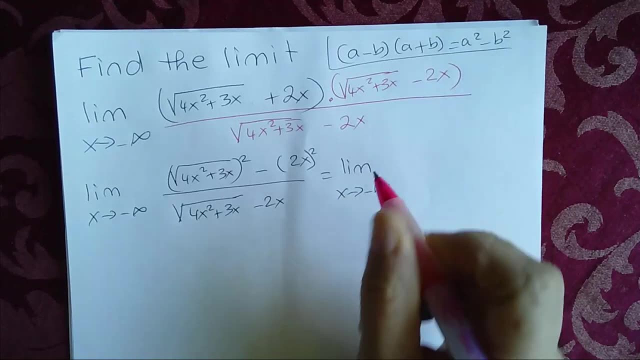 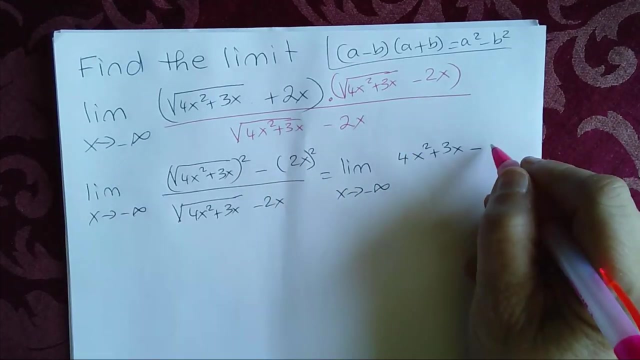 does not change. That's the limit. as x approaches, negative infinity of the square cancels the square root and you'll be left with 4x squared plus 3x minus 2x squared. that's 4x squared divided by. 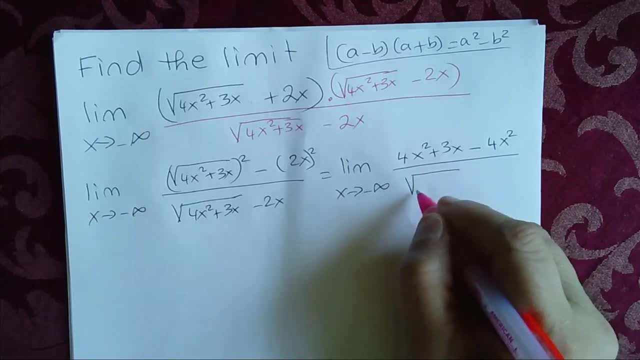 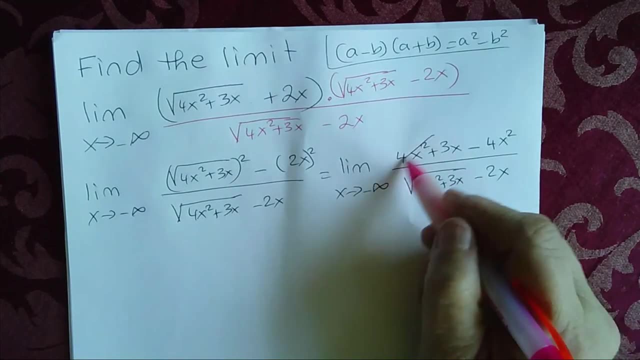 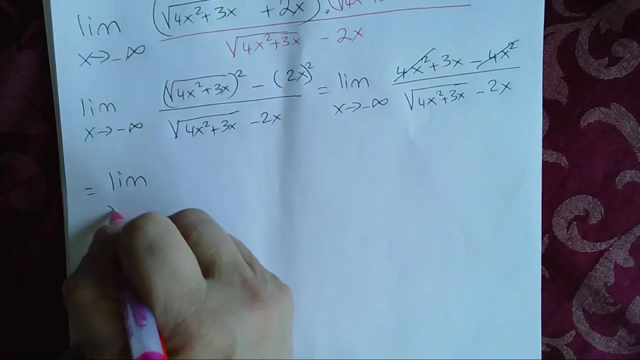 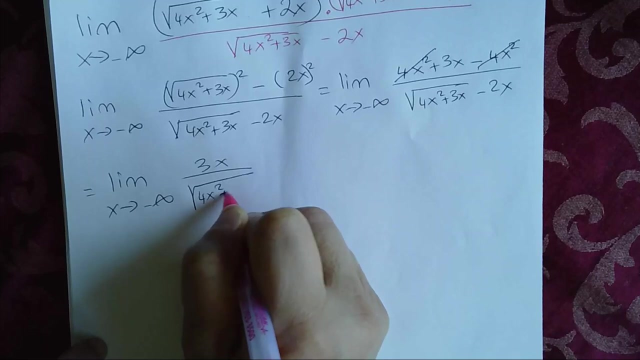 the denominator that's square root of 4x squared plus 3x minus 2x. 4x squared cancels with negative 4s squared and would be left with the limit, as x approaches negative infinity of 3x divided by square root of 4x squared plus 3x minus 2x. OK, now the variable with: 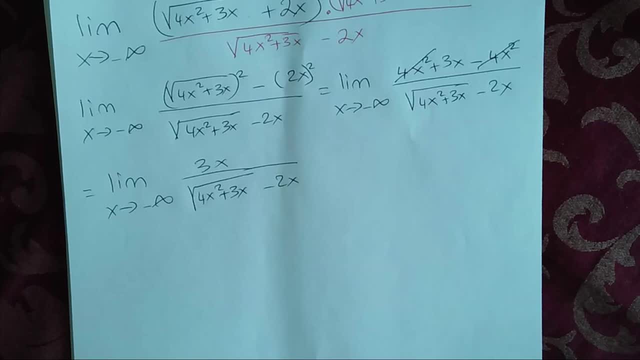 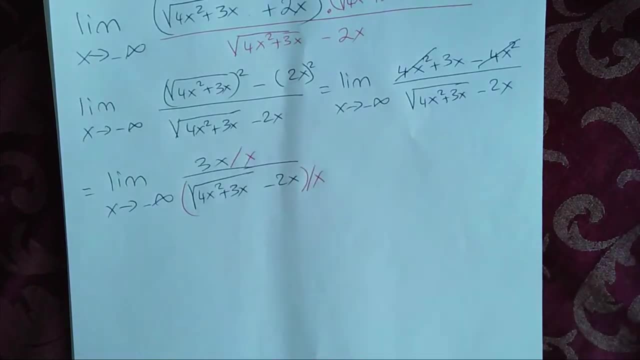 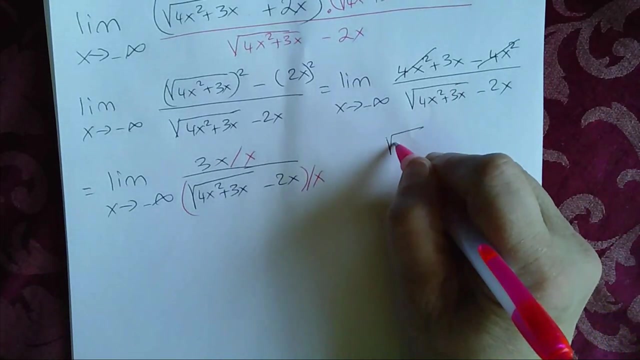 the highest power in the denominator is x. So we divide both the numerator and the denominator by x. But here we have to be careful, because when x goes inside here the radical becomes square root of x square. And what do you know about square root of x square? The square root of 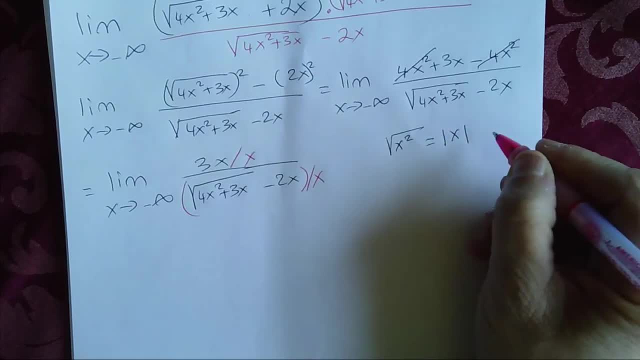 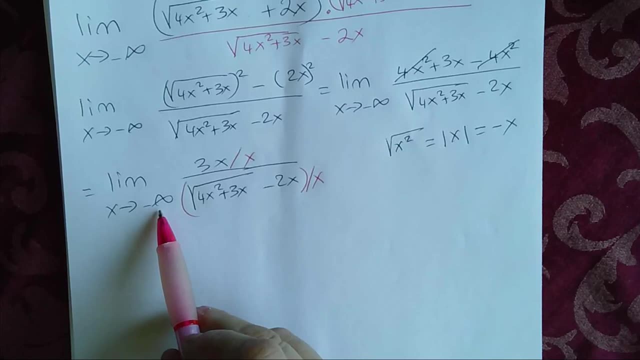 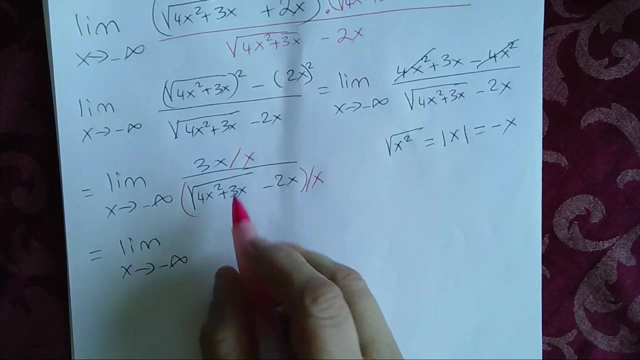 x square is the absolute value x, which is negative x. if x is negative, Well x here is negative. x's approach is negative infinity. So what we're going to get here in the next step, we're going to get: 3x divided by x is 3.. This becomes a negative because of this.